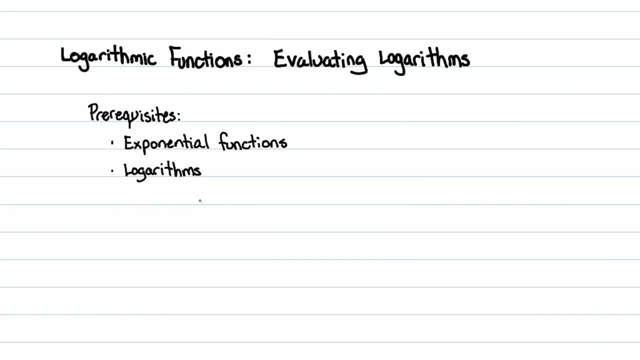 exponential functions, Not necessarily how to graph them, although you should already have done that, but everything else about exponential functions is very important. And then you should know what a logarithm is, you should know its basic use and you should also know how to transform. 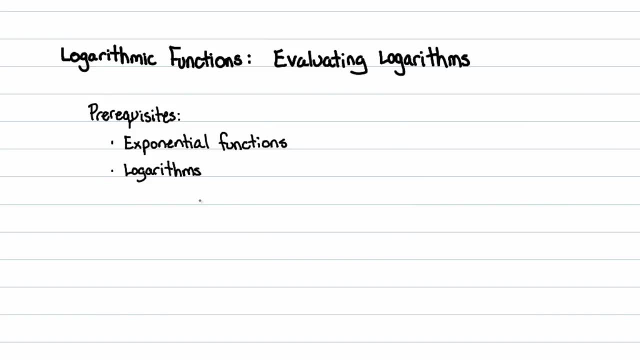 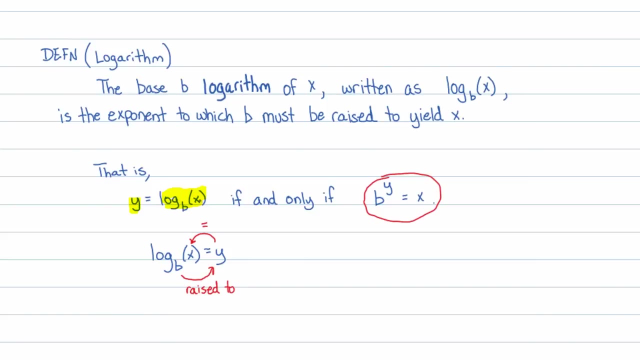 between logarithmic form and exponential form. If you don't know that, please go back one video to see my basic concepts and uses. Briefly, recall that a logarithm is just an exponent. really, The log base b of x is equal to y. 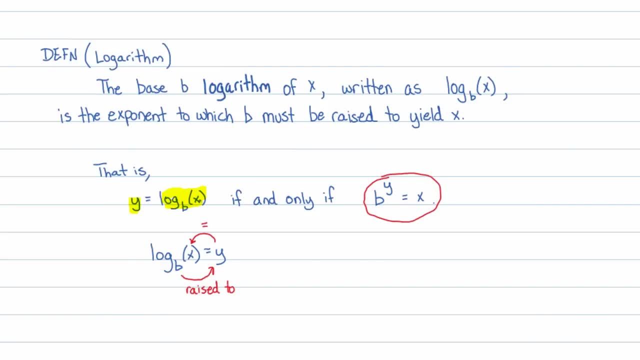 if, and only if, b to the y is equal to x, I call that my circular argument. So if this is too fast for you, like I said, you need to review my video on the concepts and basic uses of logarithms. But essentially, log base b of x equals y is the same thing as saying b raised to the y power. 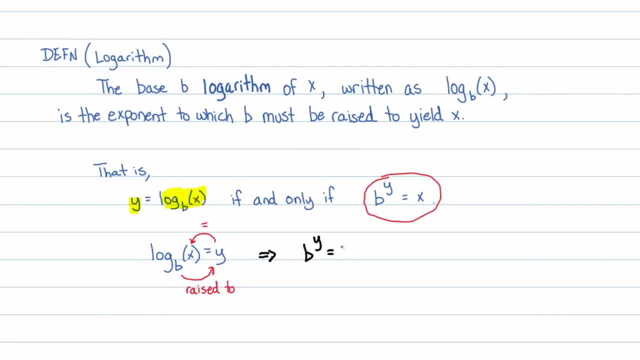 is equal to x. So let's start using this to evaluate logarithms. Now, when somebody hands you a logarithm to evaluate, it's usually not in an equation, So I'm going to delineate kind of what they gave me from what I'm going to be writing by writing in black ink for the stuff I'm adding to their 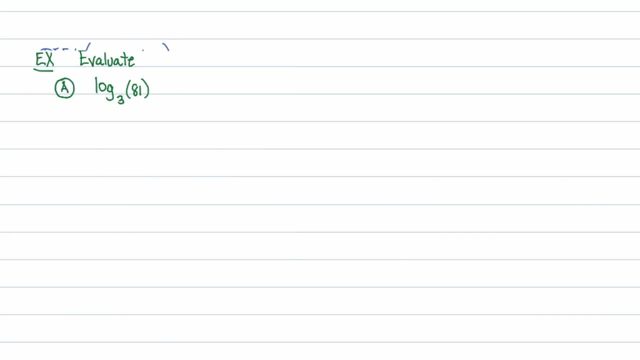 problem. So if somebody comes up and says: what's the log base 3 of 81? I usually do this- Well, I don't know, That equals some number. But then I can use this algorithm to evaluate logarithms, A circular argument now that I've written this as an equation where I say, well, it equals some. 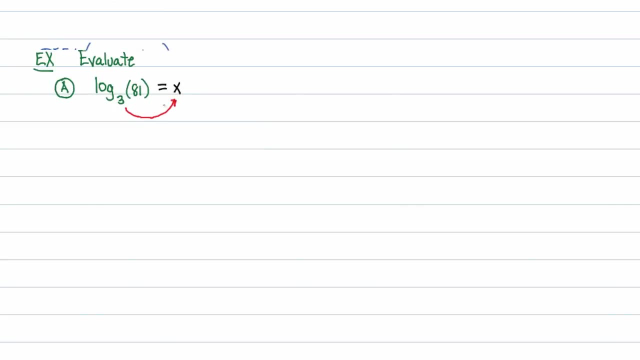 unknown. I can then use the circular argument 3 to some power. So remember this is: the raised to is equal to the inside. So this means that 3 raised to the x power must equal 81.. Now remember what we're trying to find here. We're trying to find the value of x. Well, 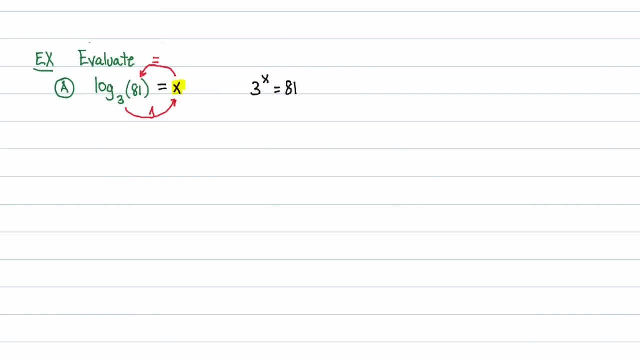 3 to 1.. What power is equal to 81?? If you're saying the fourth, you're absolutely right. 3 to the fourth, power is equal to 81. And there's a couple ways you could do this. You can either just recognize: 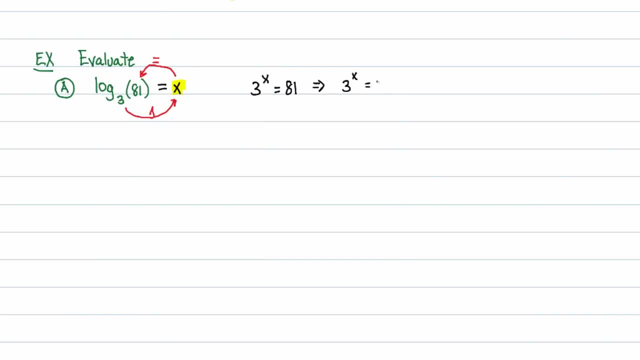 that 3 to the fourth, power is 81, or you could say 81,. well, this is the same thing as recognizing that 81 is 3 to the fourth. I'm just saying 81,. another way to write that is 3 raised to the. 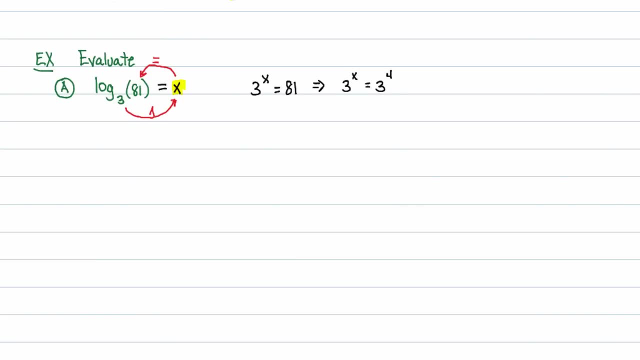 fourth power: Since these bases are the same and these exponential expressions are equivalent, that means they're exponents are the same. So I know now that log base 3 of 81 must equal 4.. Now, I was very long-winded with that, and the reason why is because I want to kind of show you every little. 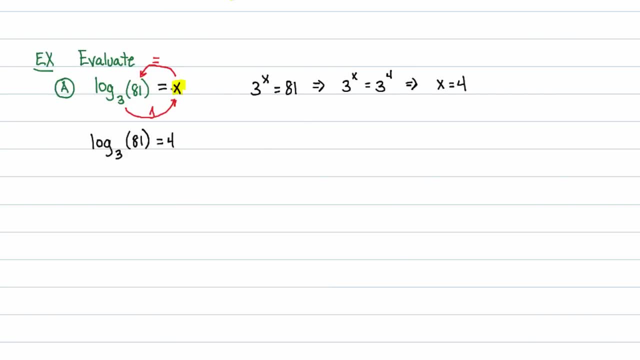 step. But really when I look at this and I always write the equals x there, I just say 3. to what power is 81? And I start thinking right. By the way, I just kind of noticed some handwriting issues. Some people might be wondering what that was. This is a caret symbol. It means raised to. 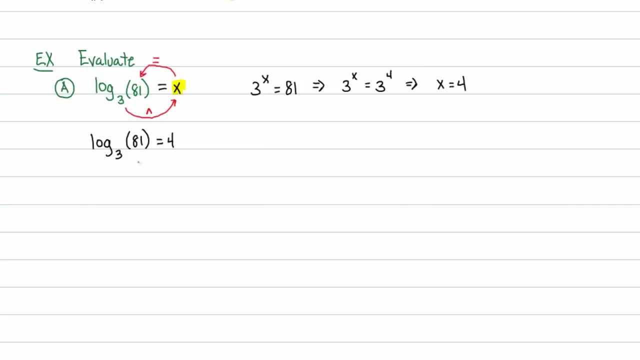 on a computer. So that's the raised to symbol I use. All right, let's try another example. Now I have log base 5 of 1 over 625.. Again, this is what they handed me. I'm going to put in here. 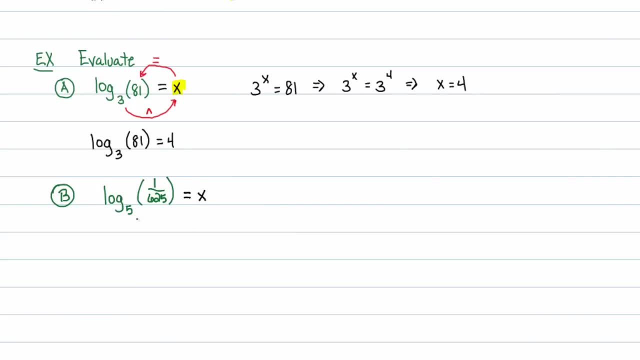 equals x, because it just makes it a little bit easier for me to see what I'm doing. So I'm going to put in here equals x And I'm going to put in here equals x, because it just makes it a little bit easier for me to see what I'm doing. So I'm going to put in here equals x And I'm going to put in. 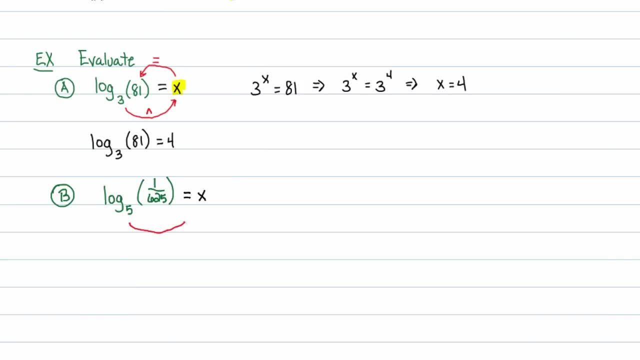 here equals x, because it just makes it a little bit easier for me to see what I'm doing. So I'm going to put in here equals x, because it just makes it a little bit easier for me to see what I'm doing. So when I use a circular argument, 5 raised to what power is going to equal that inside? So let's. 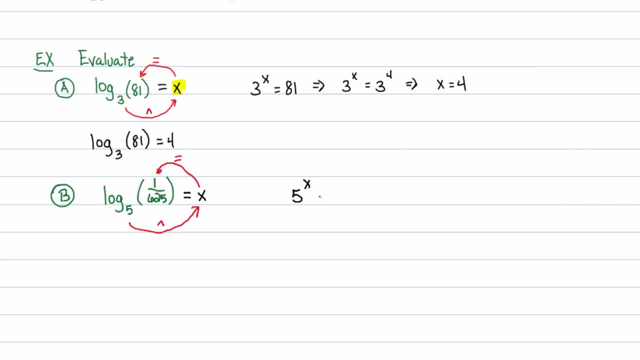 write that out: 5 raised to what power is equal to 1 over 625?. Well, you really try to write. what you should do is try to write that 625 in terms of a power of 5. It turns out. 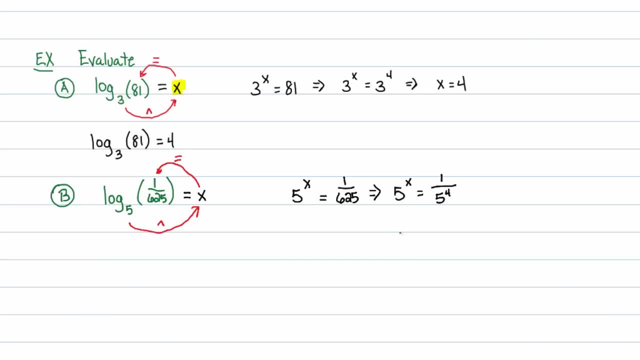 625 is 5 to the 4th power. Now notice: the left-hand side and the right-hand side are not exactly the same. The bases are not exactly the same. So I'm going to manipulate the right-hand side. I'm going to attach a negative to the exponent so I can flip that upstairs. 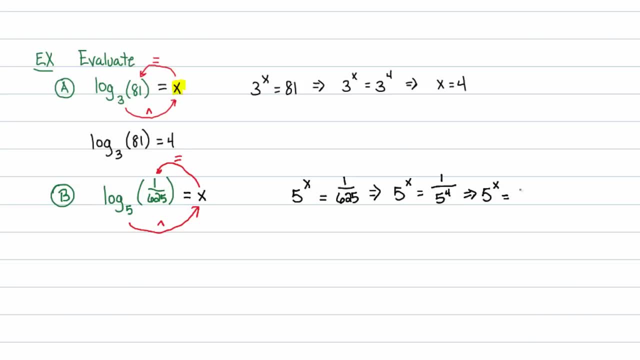 So I have 5 to the x on the left-hand side. On the right-hand side I'll have 5 to the negative. 4th Notice: their bases are the same, So their exponents must be the same. That implies x must equal a negative 4.. 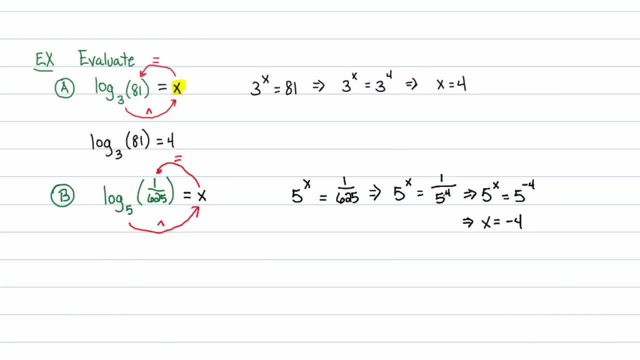 If you have a hard time with that negative exponent flipping to the top and bottom business, you should go back- probably about 20 or 30 videos of mine to find ones where I talk about negative exponents. It's a super important topic and it's an assumed prerequisite. 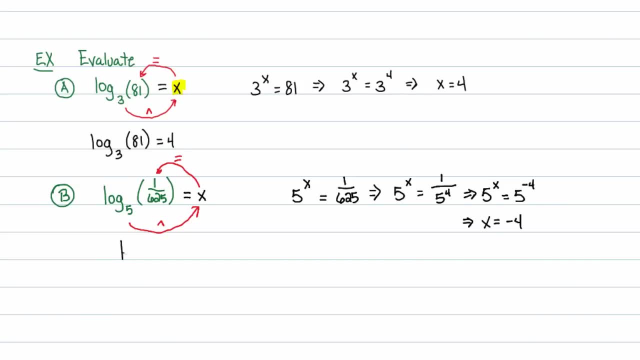 All right. so this means that the log base- 5 of 1 over 625, is going to equal a negative 4.. And you can check it out: 5 to the negative 4th power, that should equal actually 1 over something. 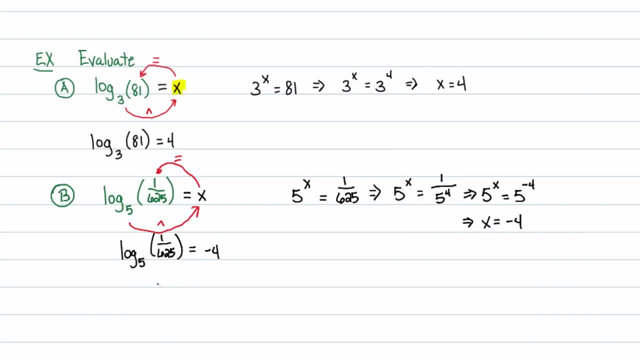 because the negative power on there means flip that 5 down to the bottom. So it does work out. Now, this one is one of my favorite examples, just because it's a great introduction to a theorem that we can use in the future, But it's a really nice problem to illustrate. 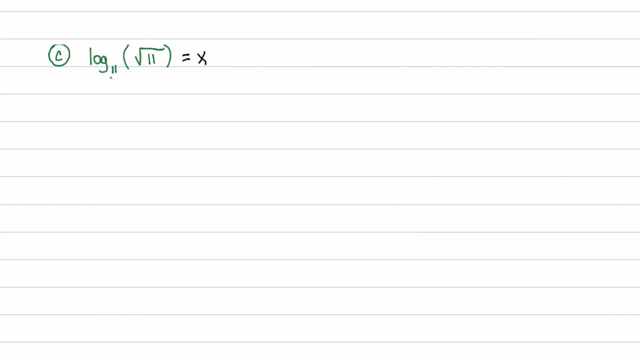 what this means. So log base 11 of the square root of 11.. And I wrote in the equals x because they didn't. It just helps me out so I can say: well then, 11 to what power is equal to the square root of 11?? 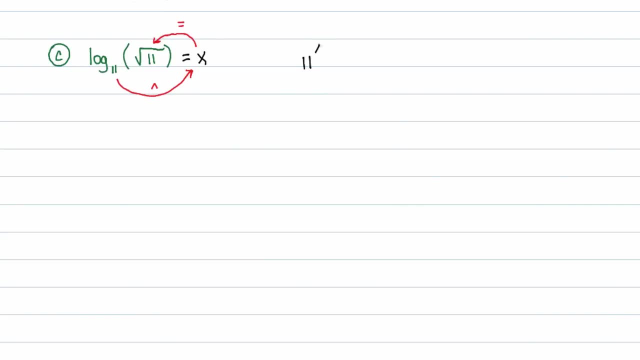 That's my question to myself. 11 to what power is equal to the square root of 11?? One thing I can do is change the square root to an exponent. right. Right, Square root of 11 is the same thing as 11 to the 1 half power. 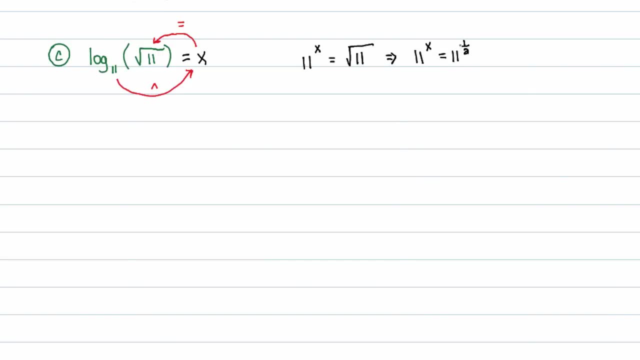 And now you see it. The base is the same, so the powers must be equal. So it means x is equal to 1 half. So what we're really saying is 11 to the 1 half. power is equal to the square root of 11.. 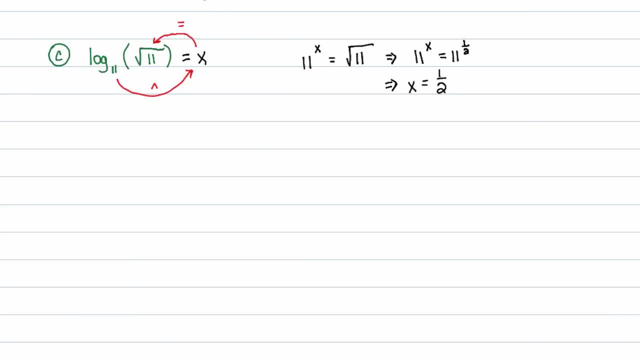 And that's absolutely true. We all know that at this point, So let's go ahead and write that down. Log base 11.. The square root of 11 is equal to 1 half. What I don't like to see as an instructor. 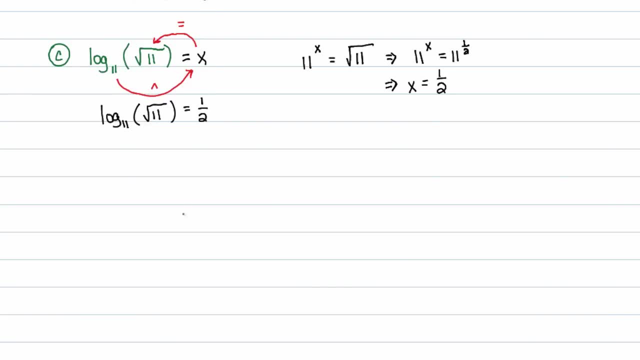 and maybe your instructor is different. I do not like you to see, I do not like you to do the following: Where you solve this all out, you get x equals 1 half and you just walk away from it. It doesn't demonstrate to me that you know what that 1 half is. 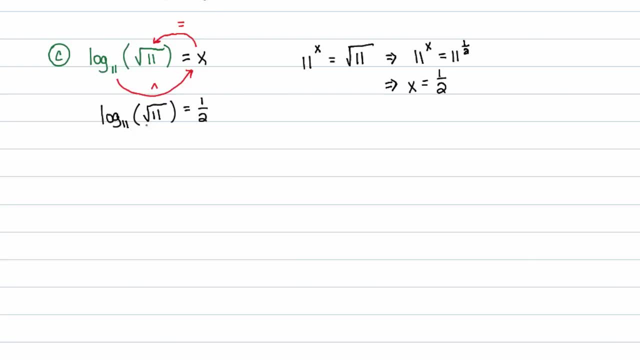 What that 1 half is. it is equal to the log base 11 of the square root of 11.. So please just rewrite this Log base: 11.. Of the square root of 11 equals 1 half And, as I just mentioned, it brings up a good indicator of a theorem here. 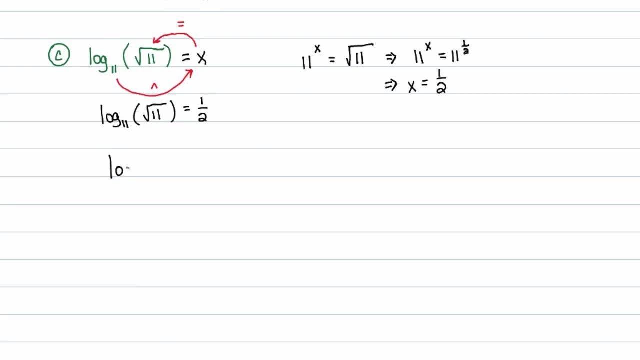 If I would have written this in exponent form first. So if I was looking at log base 11 of 11 to the 1 half power, If somebody were to ask me what's log base? 11 of 11 to the 1 half power. 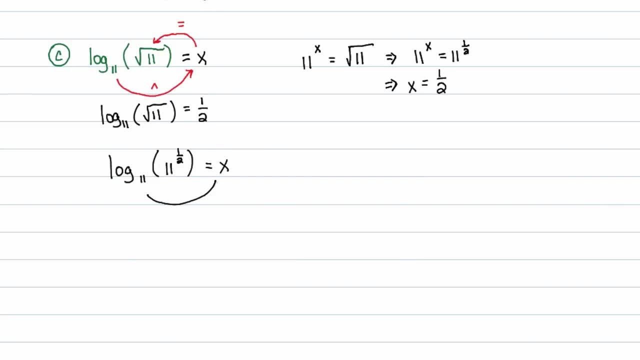 That's essentially them saying: what do I raise 11?? That's 11 minus 2 to get to 11 to the 1 half power. 11 to the 1 half would be 11 to the 1 half. So 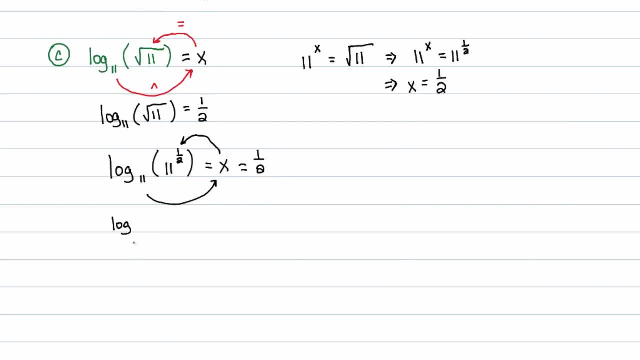 what's interesting about this is that if I had said log base- oh I don't know- b of b to the 10th power, Well, what do you think that's gonna be? B to what power is equal to b to the 10th power? 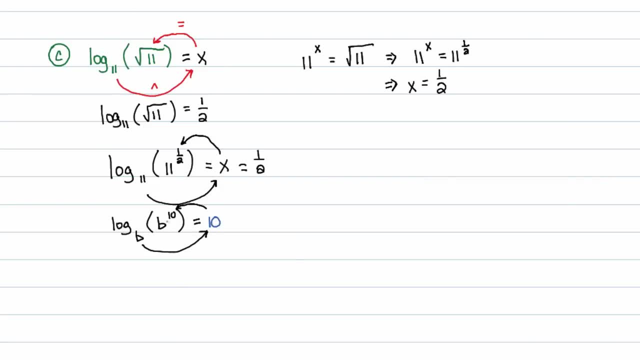 in the question 10. b to the 10th power is b to the 10th power, so this is one of the theorems that is involved in logarithms. let's go ahead and write a few of them down, given that b is not equal to 1 and b is positive, and we'll talk about why that's true in a while. 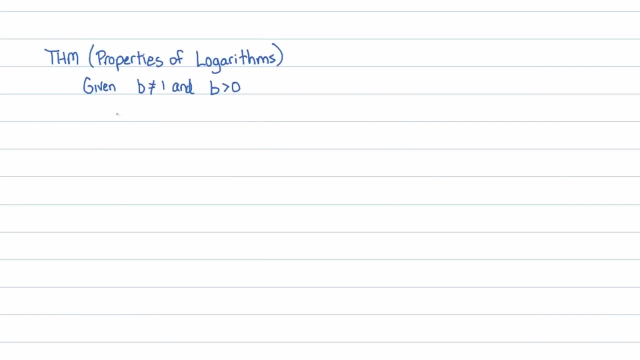 but given that b is not equal to 1 and b is positive, well log base b of b to the p power. let's ask ourselves again- i just did this problem, actually, but i had a 10 in the place of p, so let me ask you: b to what power is going to equal? b to the p power? the answer is p. b to the p is equal. 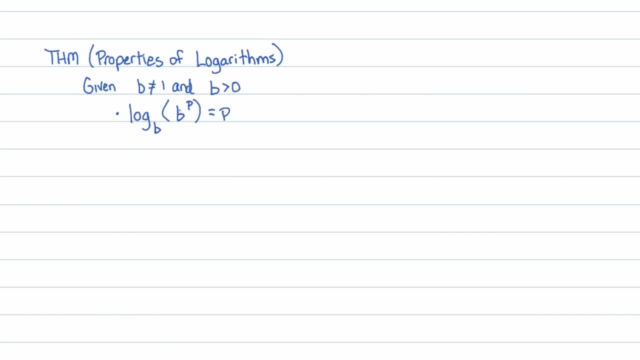 to b to p. so this theorem says: log base b of b to the p power always just going to return p. so this is always going to turn into p and, as a kind of a sub note here, log base b of b. what do you think this is going to turn into? b to? what power is equal to b? 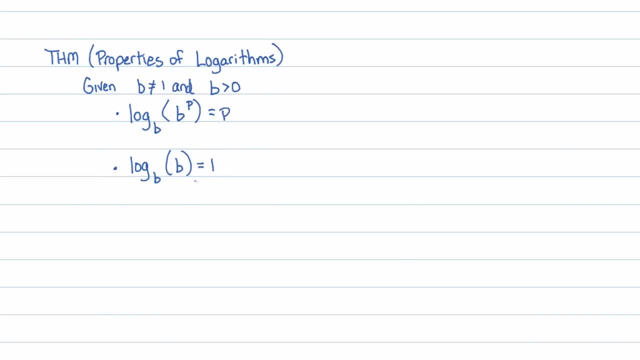 well b to the first power. so those two i consider to be the most elementary of the theorems for logarithms. there is one other one that's that's pretty neat and interesting. i guess log base b of one. this is the only one that actually really involves a number inside there. 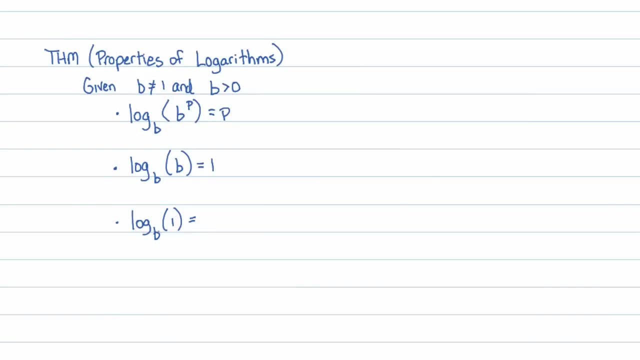 and this is the only one that actually really involves a number inside there. okay, so this is the only one that actually really involves a number inside there. b to what power is equal to one. well, let's see, you have b to some power and you know it's equal. 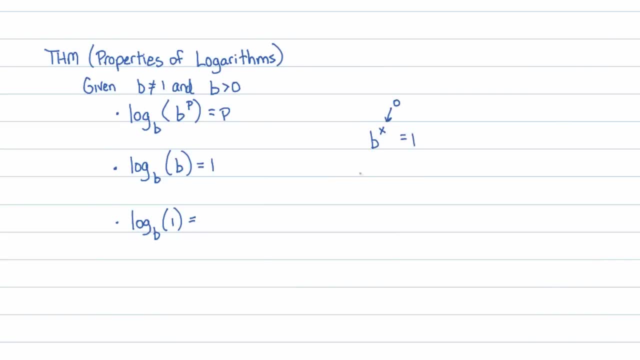 to one, that power has to be zero. b to the zeroth power is always equal to one, so this must be zero. all right, so let me erase that out, because i think i'll reuse this page in the future. that is so. these three theorems are what we're going to use for the next few problems. 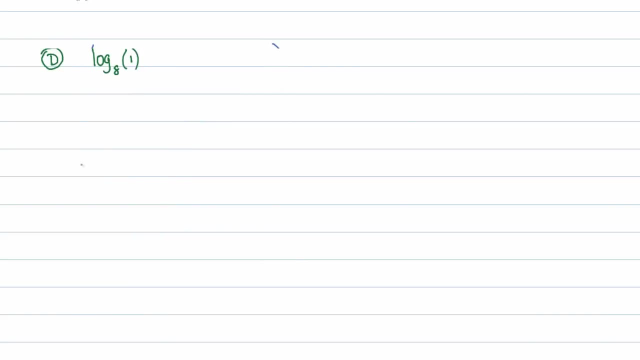 so, continuing on with our evaluations that we're at example d here, let's figure out what log base eight of one is. i don't need a theorem really to tell me what this is, because i know eight to what power is equal to one. well, eight to the zeroth power is equal to one right circular argument. 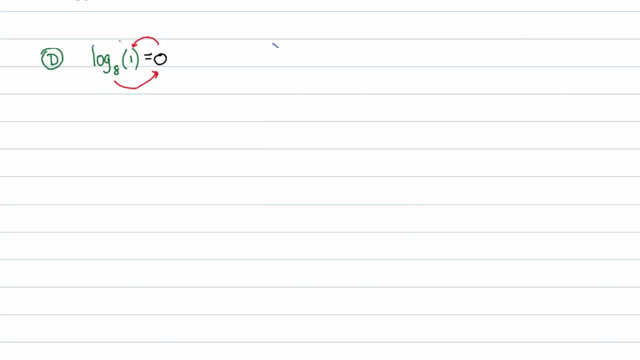 eight raised to the zero is equal to one. so that was a pretty fast problem. and and those three first three theorems are the same thing. so let's see what we're going to do here. how about the log base? one point one, two of one point one two. now i i like this problem because 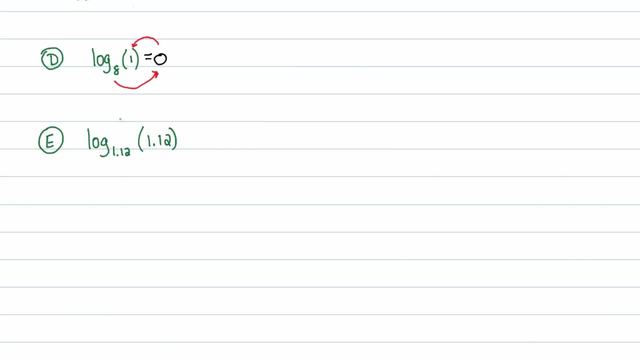 it demonstrates that logarithms do not have to have just pretty looking bases. they can have decimal bases or fractional bases as well. so one point one two to what power is equal to one point one two. one point one, two to the first power. so what power is equal to one point one two. one point one, two to the first power. 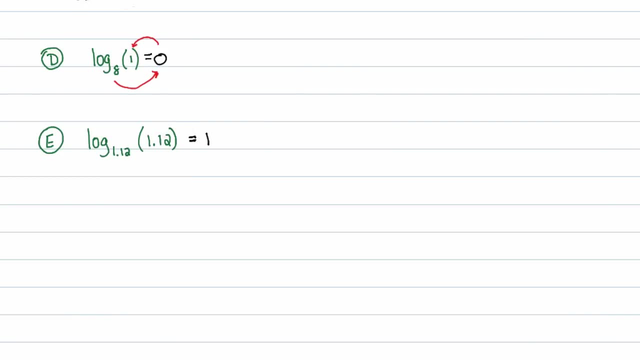 is equal to one point, one, two, so that's again using a circular argument. okay, so there we go. now let's make it fun and i highly encourage you to pause these videos. every time you see an example, pause it. try to figure it out. this example is called a nested set of logarithms, and you follow. 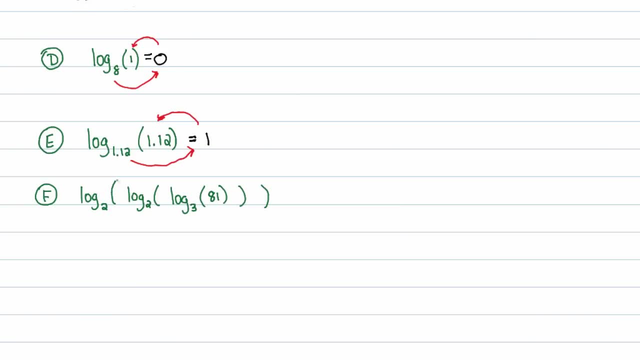 the order of operations always. so you look inside the innermost parentheses. here the innermost parentheses are the order of operations and you follow the order of operations always. so you look inside the innermost parentheses. here the innermost parentheses actually is going to be this: 81. 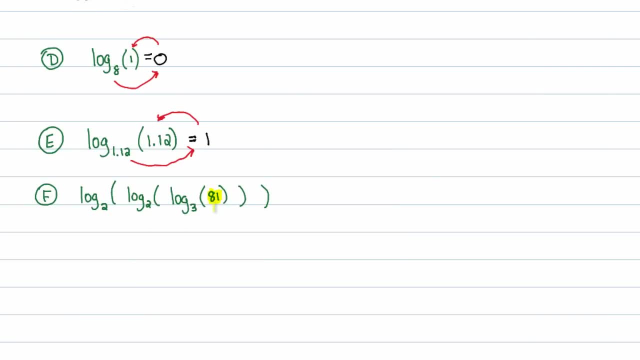 right, and you can't really simplify 81, so now you focus on the next set of parentheses, innermost parentheses, this group right here. and i know what the log base 3 of 81 is actually. let me write it above. log base 3 of 81 is just some number. well, three to what power is 81? well, three to the fourth power, three to the. 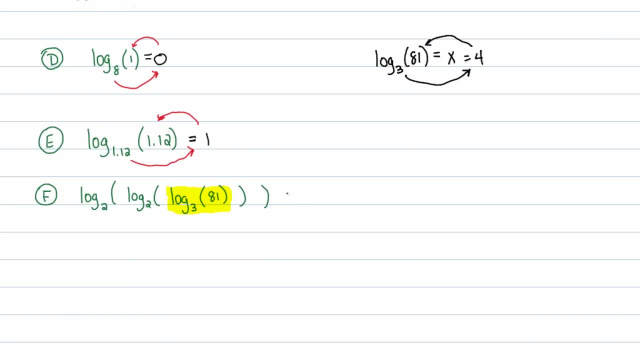 The fourth power is 81. So I know that this is just going to equal the log base 2 of, the log base 2 of, And then, instead of log base 3 of 81, I'll replace it with 4.. Again, follow the order of operations. 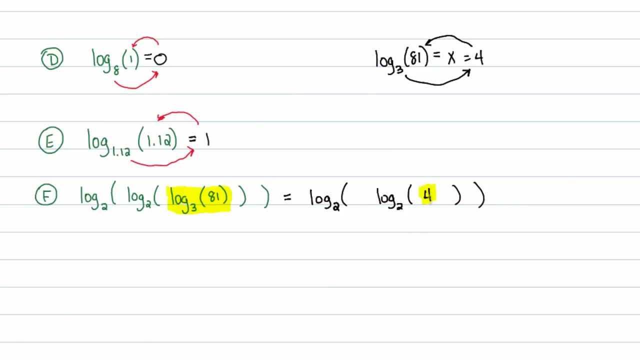 I look on this innermost parenthesis. here There's nothing to simplify, So I go ahead and focus in on the next set of innermost parenthesis: Log base 2 of 4.. And again, I'll just as an aside, log base 2 of 4.. 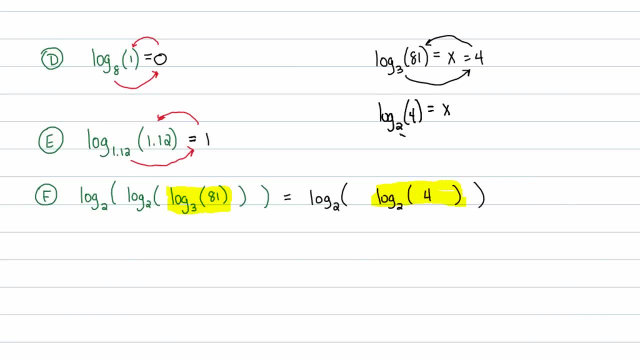 Well, let's see: 2 to what power is equal to 4?. 2 to the second power is equal to 4.. So this highlighted section right here should just turn into the number 2.. So this is going to be log base 2 of, and then 2.. 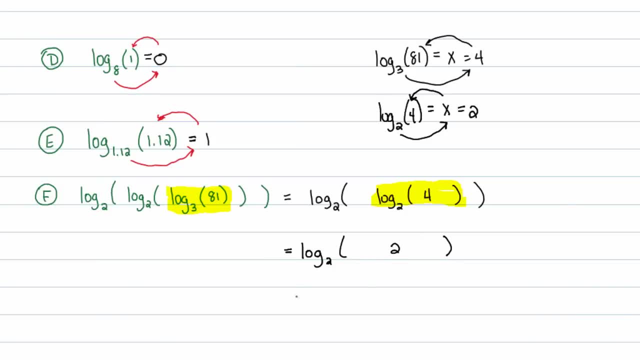 Now I know. So 2 to what power is 2?? Well, this is just 1.. 2 to the first power is 2.. There we go, And also, by the way, I am using this previous theorem here to do: 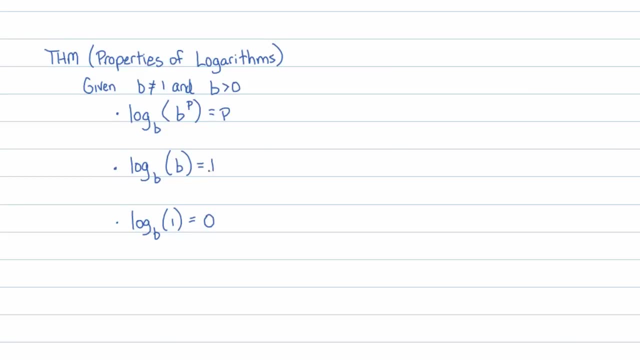 You could use this previous theorem: Log base 2 of 2 would be 1.. Or you could just use a little bit of logic. I like the logic part of it. Now it turns out certain bases are more popular to use with logarithms than others. 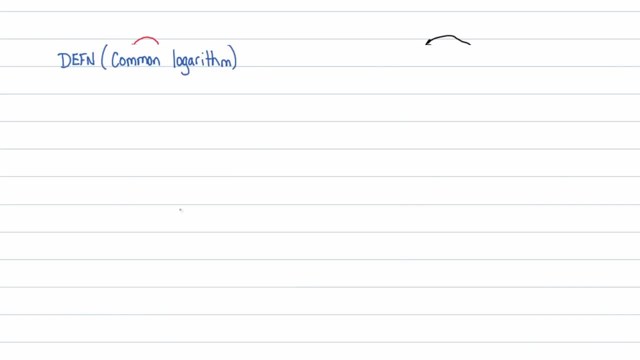 Okay, If you had to use log base 3,, log base 7, log base 24, log base 1.12 all the time, your calculator would need a button for each of those bases. Well, I mean, if there was no way to convert. 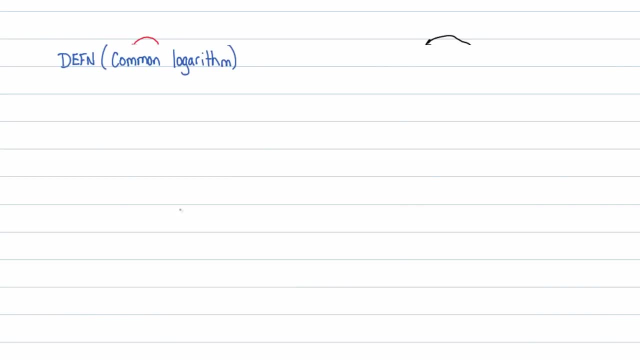 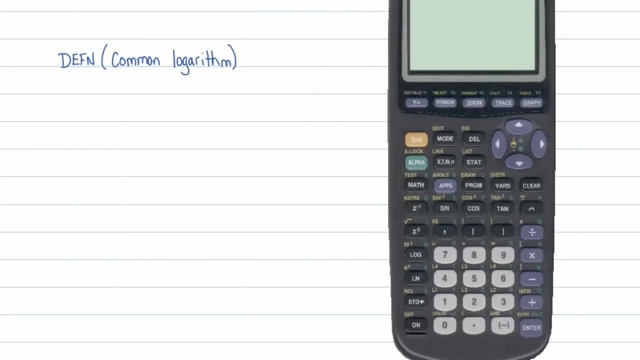 But let's just pretend your calculator would need a button for all those bases. If you look at your calculator, though, you likely- well, maybe I'll bring up mine- you likely only have a single button for the logarithm. It just says LOG, and it doesn't give you a base on it. 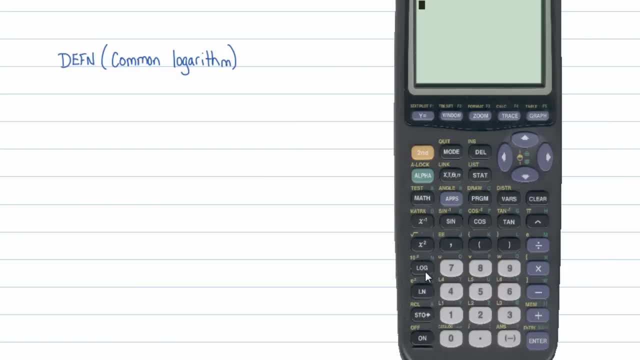 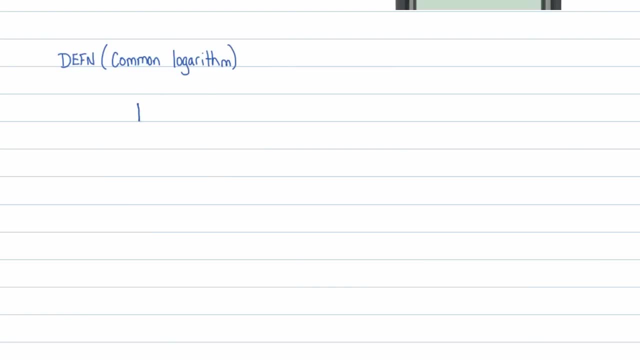 A lot of students might think: well, what would I do with that? Do I just tell it what the base is? And the answer is no. actually, It turns out that log base 10 is such a common base for a logarithm, the 10 bases. 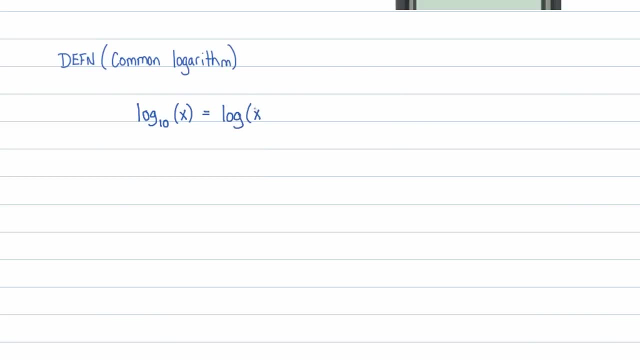 that they often just rewrite it as log of x. So if you see somebody write something as log of x or log of 10 or log of 28 or log of 357, and there's no base written down, it's implying that the base is 10.. 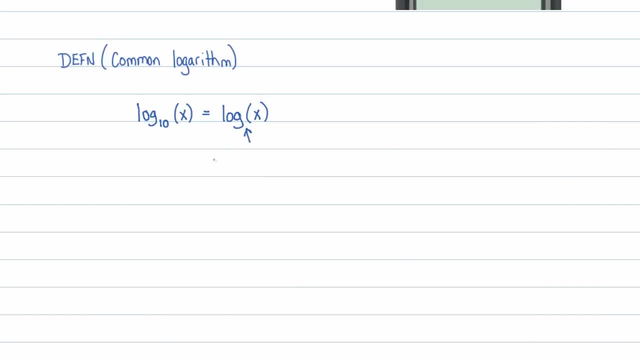 Okay, it's like the lazy man's base, but the best type of base to use. actually, Log base 10 is a really good base to use. It's so common that we call it the common logarithm. All the rules still hold for the common logarithm. 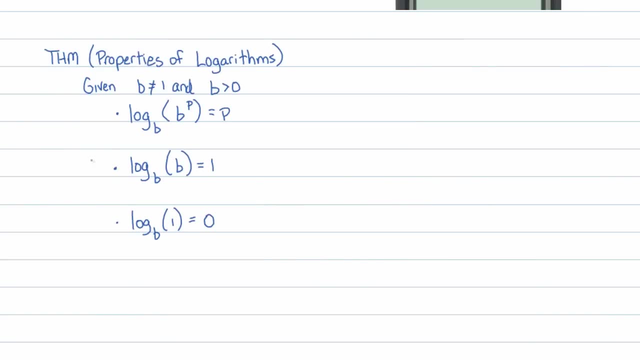 So all these theorems that we talked about right here hold, if this is just a 10 down here. So log base 10 of 10.2.. 10 to the p power, it's just p Log base 10 of 10, 1.. 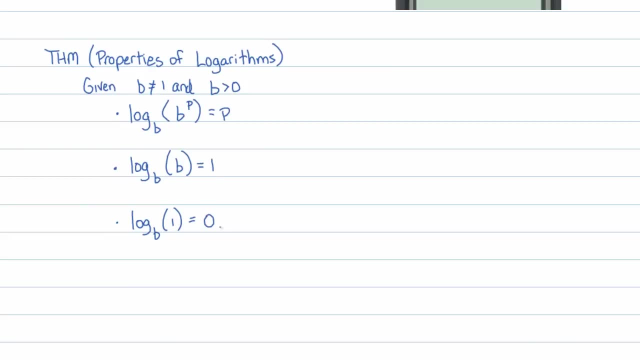 Log base 10 of 1, 0.. So, continuing on with our evaluation set of examples, here let's look at what log of 100,000 is This you could do by hand. You just have to rewrite this a little bit. 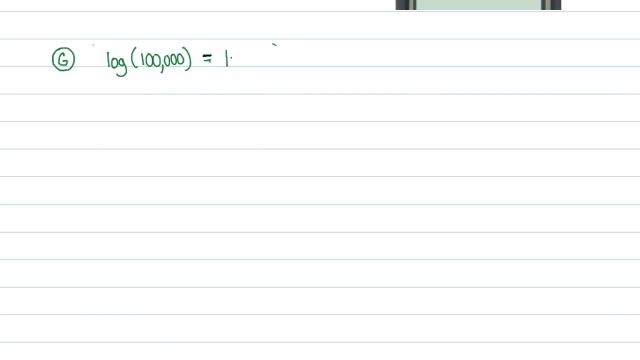 Oops, I was supposed to be writing this in black, because this is what I'm adding on Log of 10 to the something Power. What is 100,000?? Well, let's see, Count up the zeros: 1,, 2,, 3,, 4, 5.. 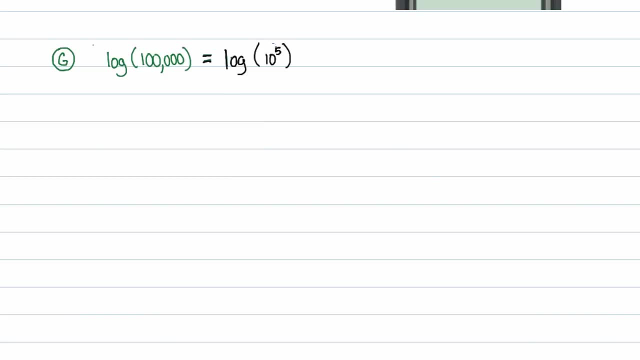 That's 10 to the 5th power. Now, remember, if I haven't written a base, you can assume that it's log base 10.. That's log base 10 of 10 to the 5th power, which will turn into 5, because 10 to the 5th is 10 to the 5th. 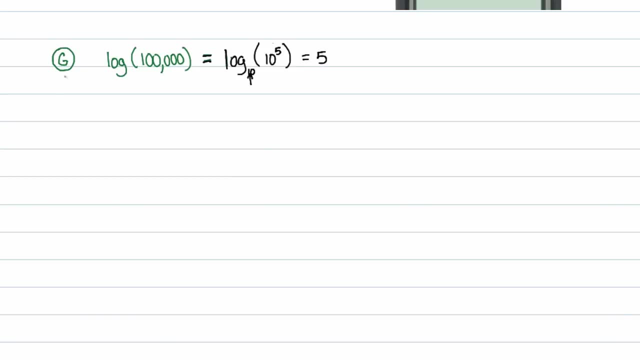 Get it. Let's try another one. Let's try. I'll just make this one up: Log of 0.0001.. Again, I know that the silent base means it's a log base 10.. And I would really like to write this as a power of 10, if I can. 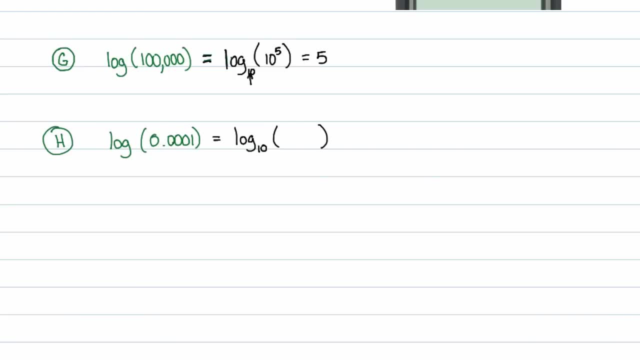 If I can't then I will not. But as I see it right now, this is a power of 10.. It's 10 to the negative- some odd power. So let's see, That's 10 to the negative. 4th right: 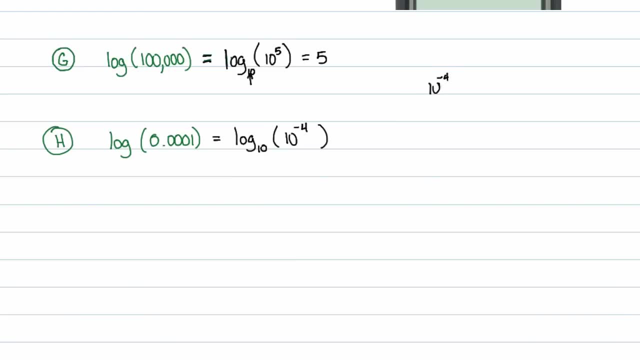 You can check that. by the way, 10 to the negative 4th is just 0.1234.. Yeah, so that is 10 to the negative 4th. So I have log base 10 of 10 to the negative 4th. 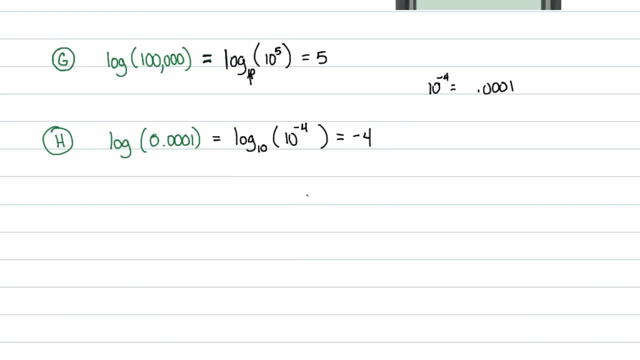 This will turn into a negative 4.. Now, it's not always going to be the case that somebody hands you a log base 10 of a nice pretty number like this. These are both powers of 10.. The question is what happens if you don't have a log base 10 of a number? that's a power of 10?. 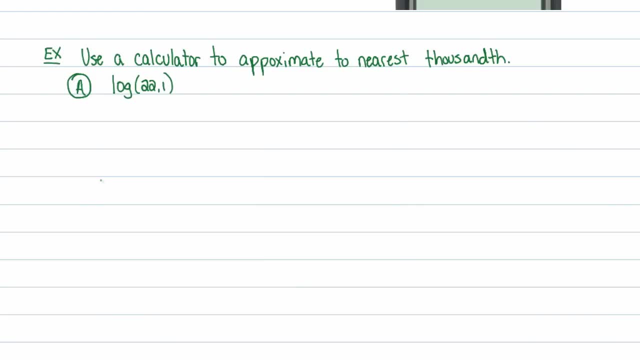 For example this- This is the more common case- That you have log of 22.1, which again is just log base 10.. You don't have to write it in there, I'm just kind of showing you that it is log base 10 of 22.1.. 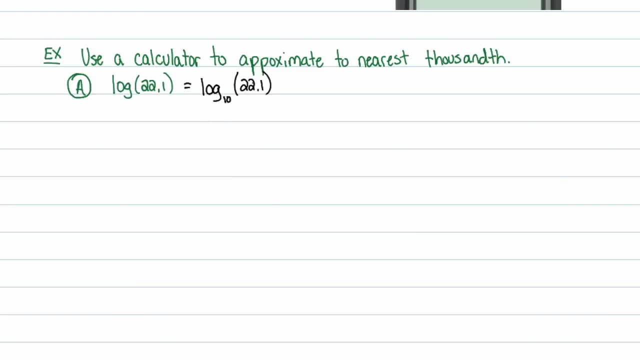 And so now the only way to find out what this value is is to write it in there. And the value is: because 22.1 is not a nice power of 10,. what you're going to need to do is grab a calculator. 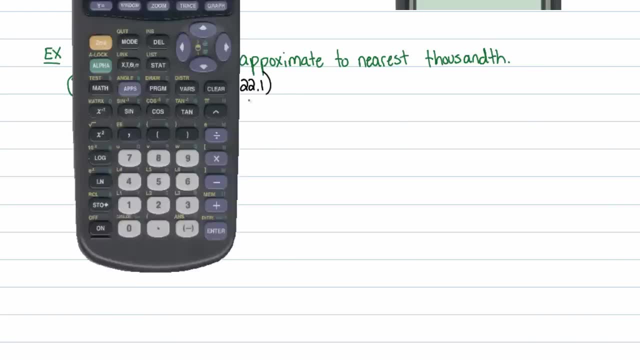 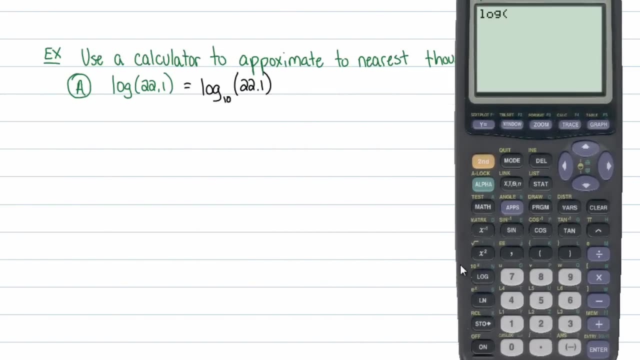 And it does tell you in the problem to grab a calculator and round to the nearest thousandth anyway. So let me go ahead and do that On a calculator. you just hit the log button. It automatically knows you mean base 10. And type in 22.1.. 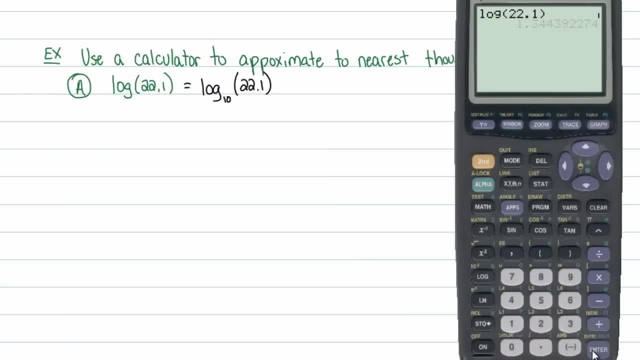 You don't really have to end parentheses, but I do. That's 1.344, roughly, And if you're using some type of, if you don't have a calculator with you, you can always use the internet. Using the internet, and I guess I didn't need to leave the calculator up, but I did.